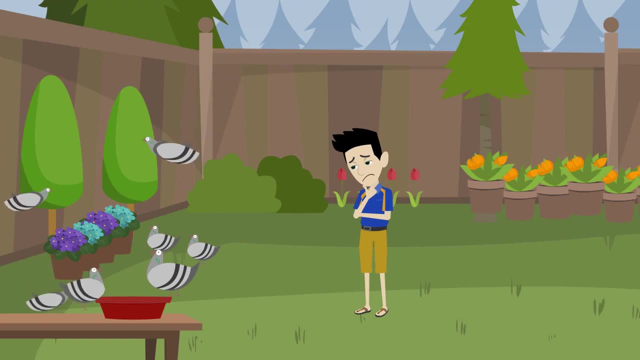 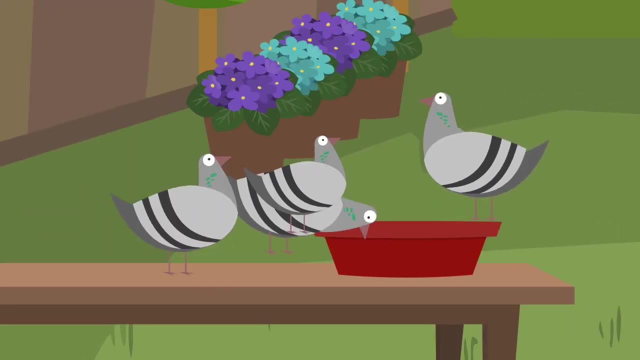 Viraj was still in the garden when few birds came to drink water in the pot where they used to keep water for the birds. Viraj looked at them and became aware They were sad as it had no water. The birds searched here and there for water. 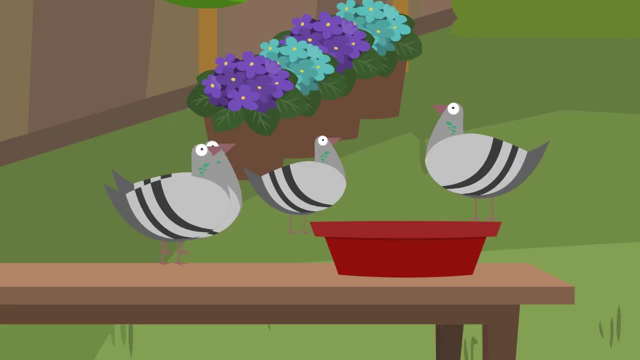 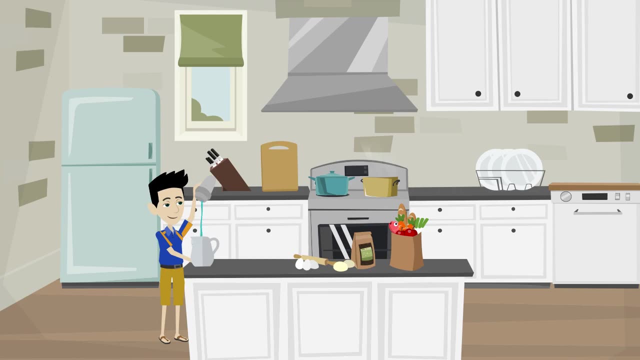 Viraj began to realize that he had to water the plants. He realized his mistake and went inside the house to arrange some water. As they didn't have any water in the house, Viraj poured some water from his bottle in the fridge and kept it for the birds to drink. 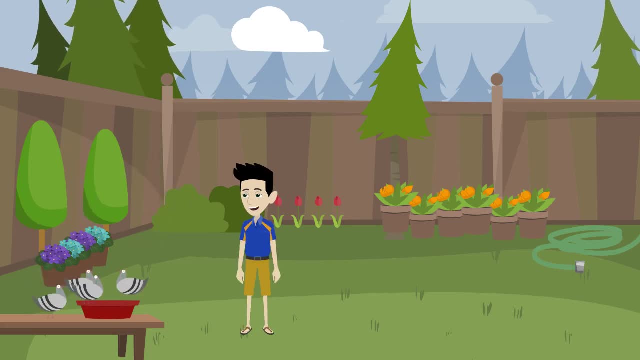 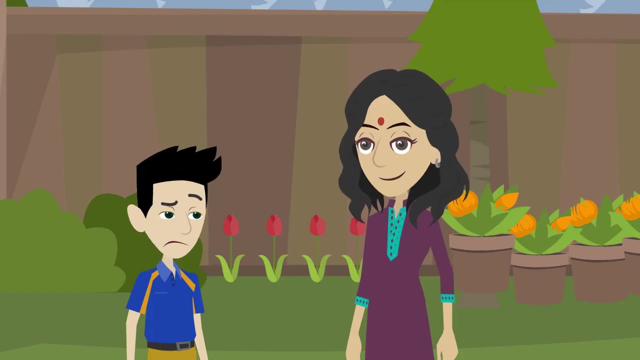 The birds drank the water. They chirped happily and flew away. Viraj was happy too. He looked back and found his mother standing there. He accepted his mistake and said: Sorry, Ma, I will not waste water again. He looked back and found his mother standing there. He accepted his mistake and said: Sorry, Ma, I will not waste water again. 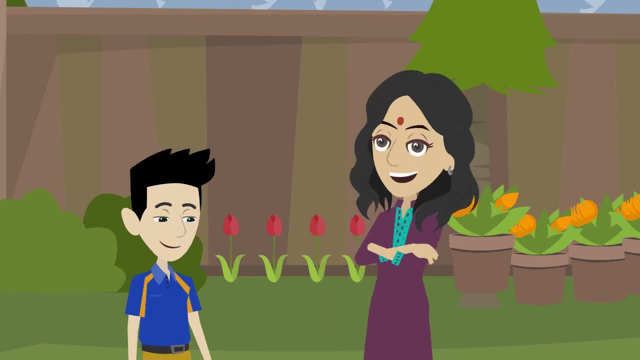 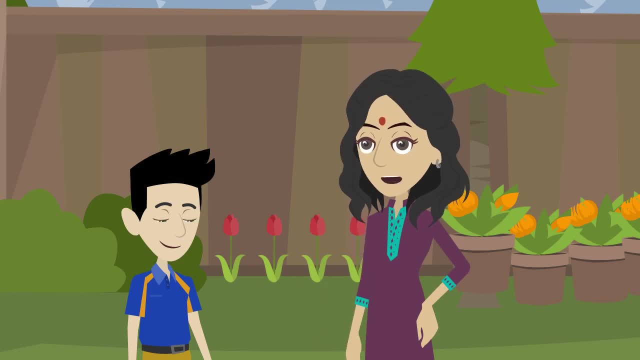 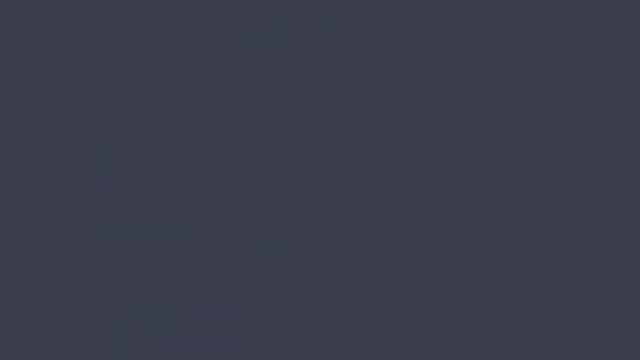 Good, You realized your mistake. Water is very scarce, Pita, So we must use it properly. Good, You realized your mistake. Water is very scarce, Pita, So we must use it properly, it properly, otherwise we will also become thirsty, like the birds. moral of: 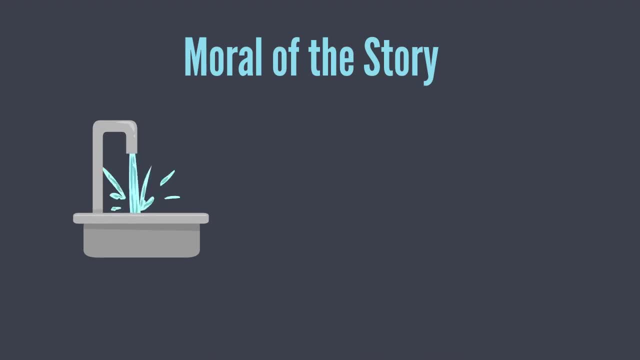 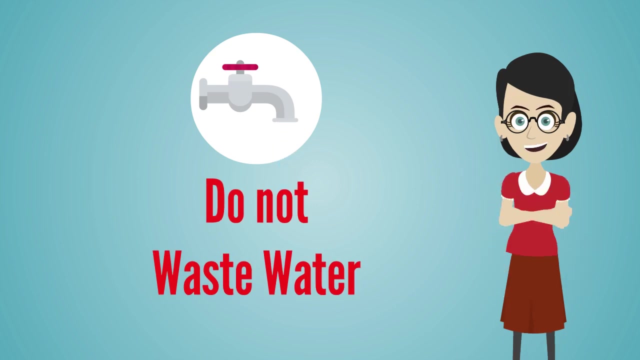 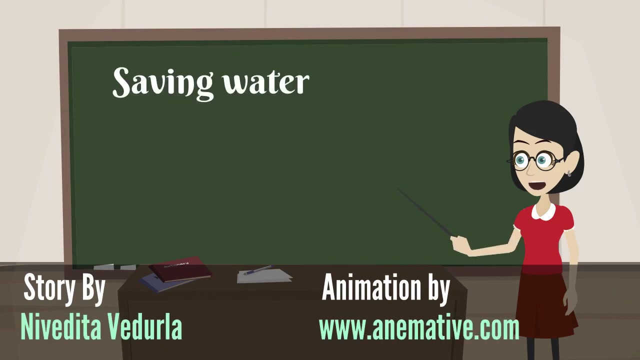 the story is water is rare and becoming less. if we don't use water properly today, then tomorrow we might not get it even to drink. so, kids, we should not waste water and stop others from wasting it. to save water, save nature. so, kids, today we learned about saving water, helping others and always listen to your 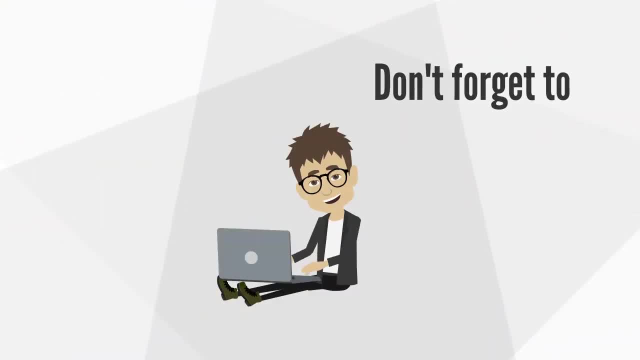 elders, kids. if you enjoyed watching this video, do like and share with your friends, and do not forget to click on the red color subscribe button below the video and stay tuned for more such amazing videos.